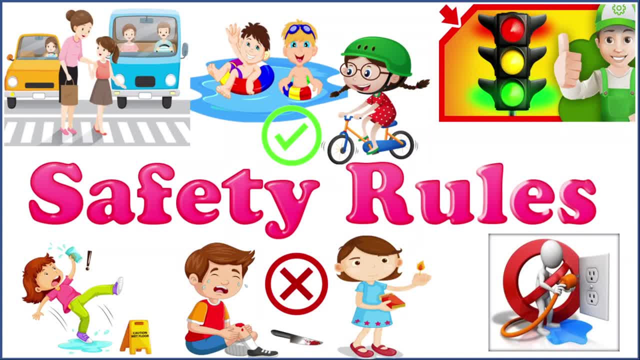 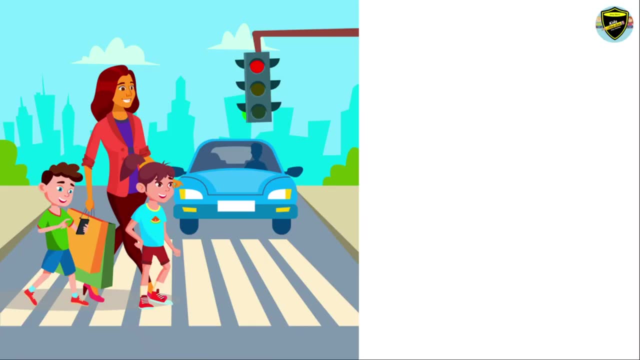 of how to tackle a particular situation, And for this, knowledge and awareness is very important. So watch this video thoroughly. It will definitely help you. First of all, we will focus on safety on road. While we are at road, always make sure. 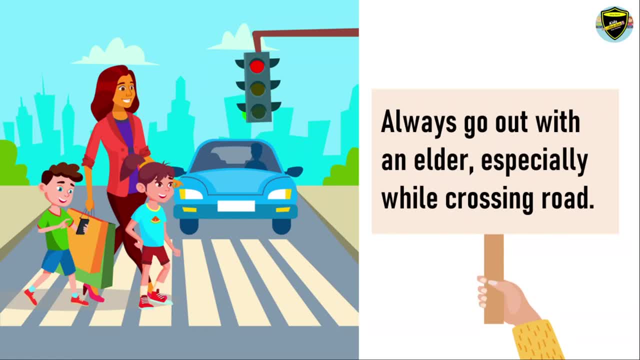 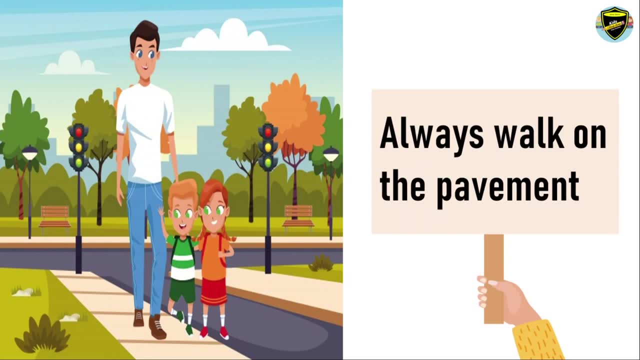 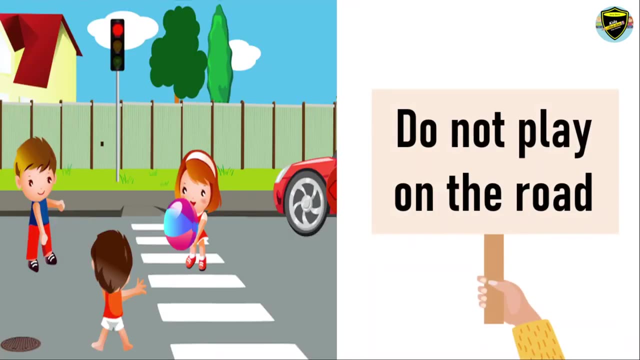 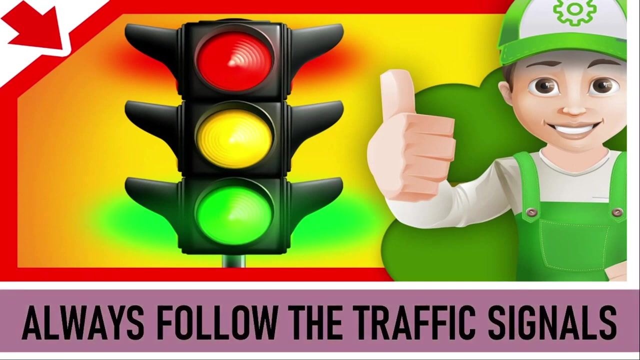 Always go out with an elder, especially while crossing the road. Always walk on the pavement. Always cross the road at zebra crossing. Do not walk on the pavement. Do not play on the road. You may hurt yourself. Always follow the traffic signals. 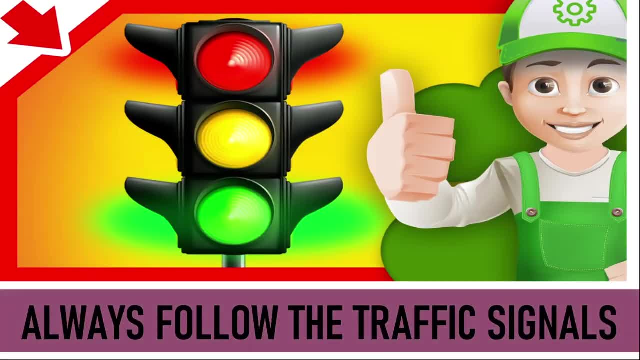 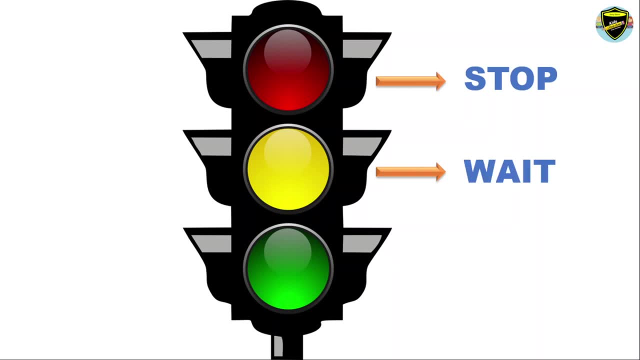 Now let us see what the traffic light says. The red light says stop, The yellow light says wait And the green light says go. Children always remember: if we follow these traffic signals, we can do our duty well. 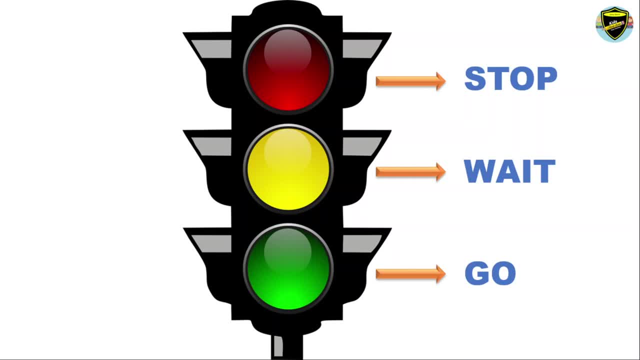 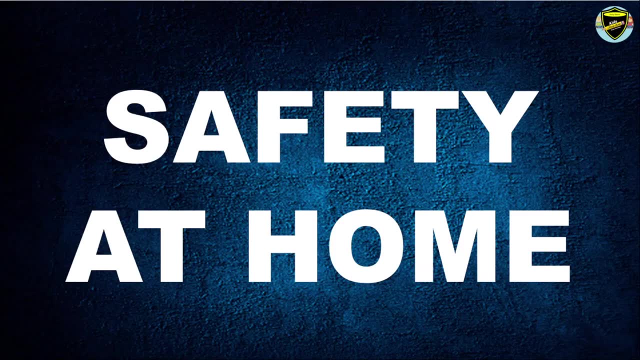 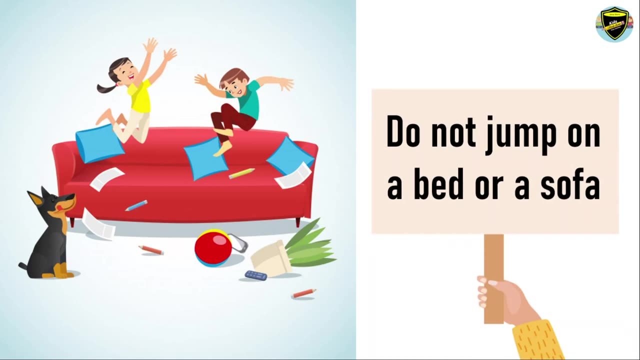 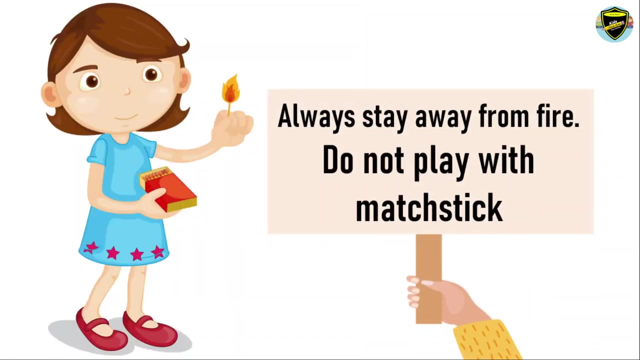 Always remember. if we break these traffic rules, we will put others also into trouble. Now let us focus on safety at home. Do not jump on a bed or a sofa. If you happen to fall, definitely you will get injured. Always stay away from fire. Do not play with match. 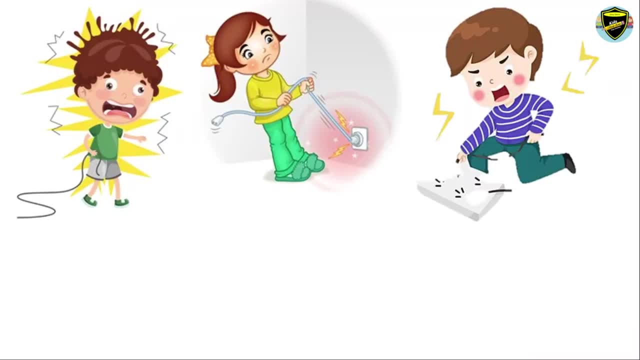 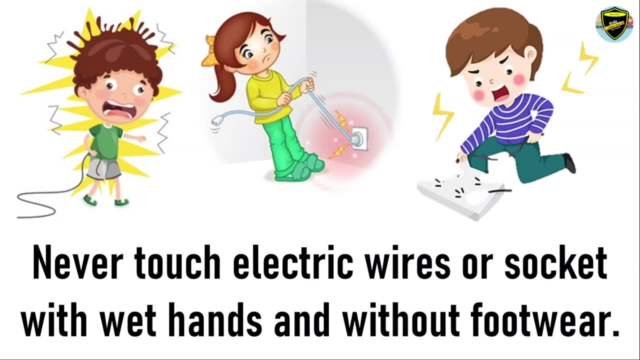 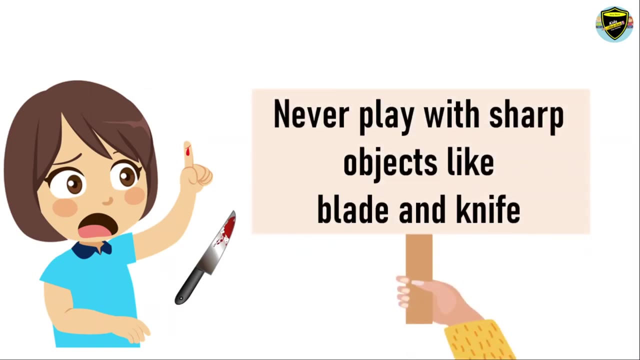 sticks, You may burn your finger. Always stay away from fire. Do not play with match sticks. You may burn your finger. Never touch electric wires or sockets. with wet hands and without footwear, You may get electric shock. Never play with sharp objects like blade and knife. Remember children. you may cut your finger. 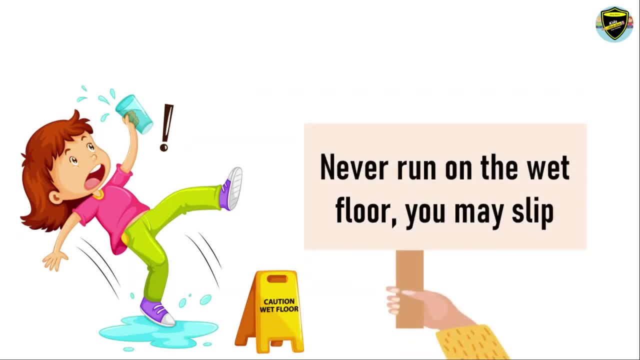 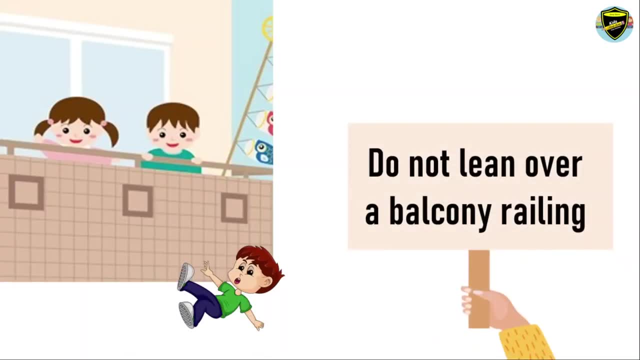 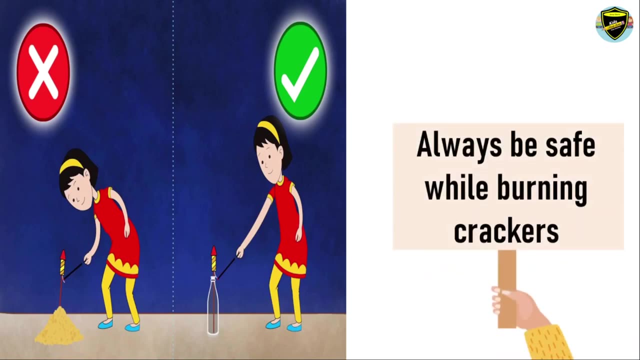 Never run on the wet floor You may slip. Never run on the wet floor You may slip. Do not lean over balcony railing. Chances of accident are more. Always be safe while burning the crackers. It will be very good if you do this in presence of elders. 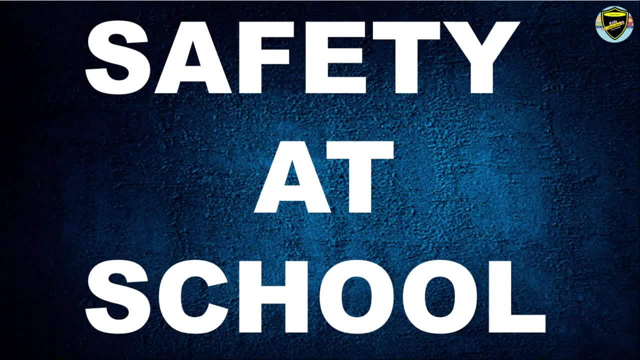 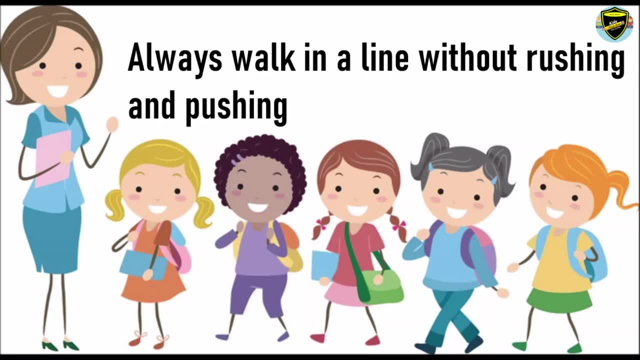 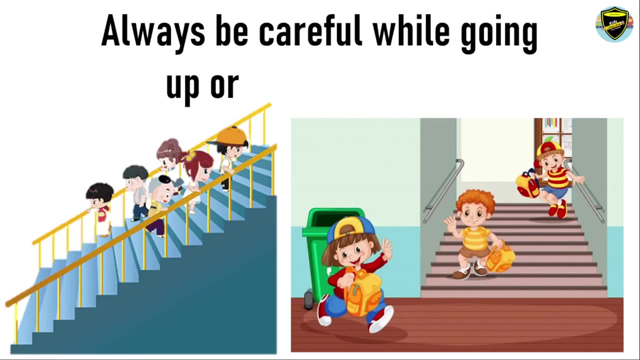 Now let us see what all are the safety we need to keep in our mind while we are at school. Always walk in a line With rushing and pushing. In this way, we can save ourselves as well as others from falling. Always be careful while going up or down the stairs. Running fast can make 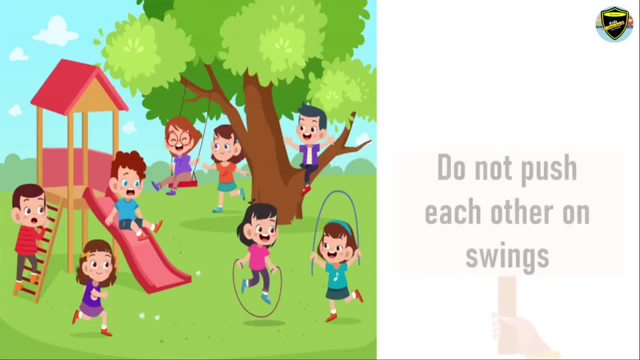 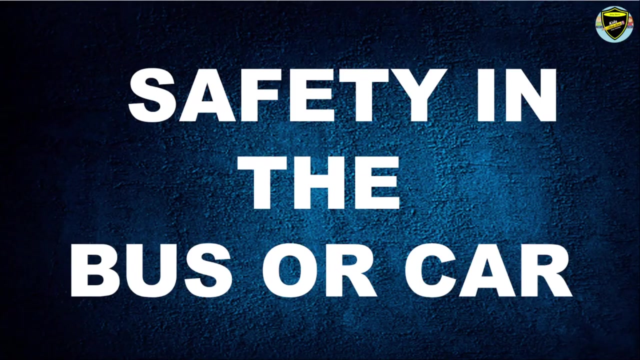 accidents. Do not push each other on swings, Take turns and play very safely. Do not harm anybody. Do not jump on the chairs and desk. Now let us focus on the safety measures we need to keep in our mind while we are travelling in a bus or a car. Remember children always. 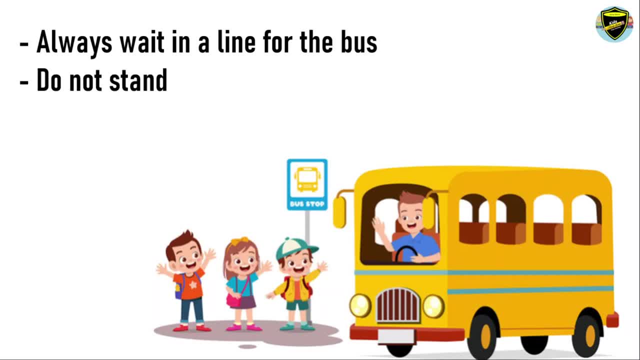 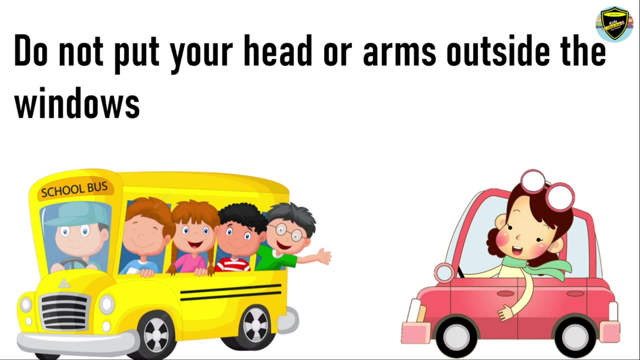 be careful while going up or down the stairs. Always be careful while going up or down the stairs. Do not stand near the door of the bus. You may fall. Never disturb the driver. It distracts the driver and leads to accidents. Do not put your head or arms outside the windows. 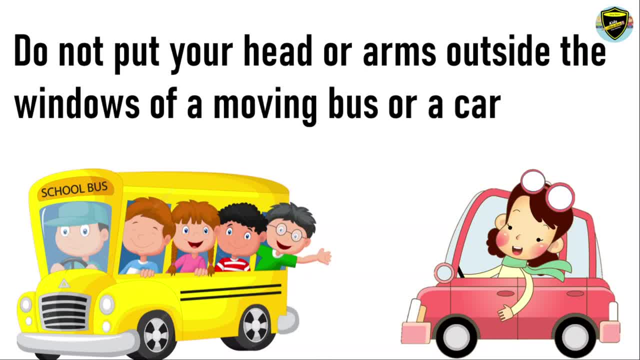 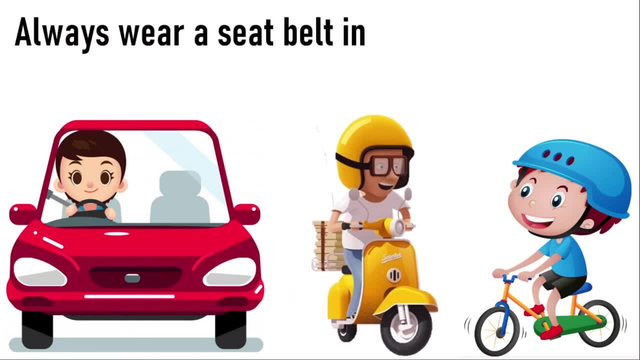 of a moving bus or a car. Remember children. always be careful while going up or down the. Remember you may hurt yourself. Always wear a seat belt in a car and a helmet while driving a two-wheeler. Now let us focus on the safety while we are in the pool. 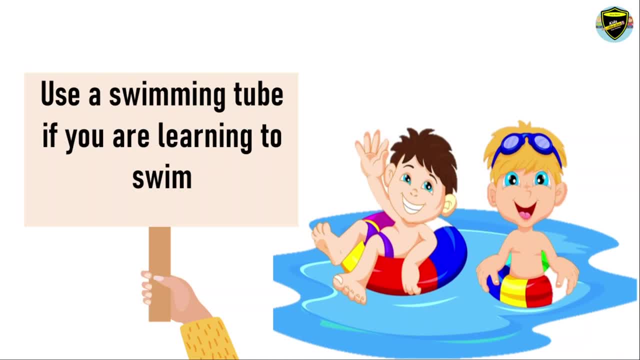 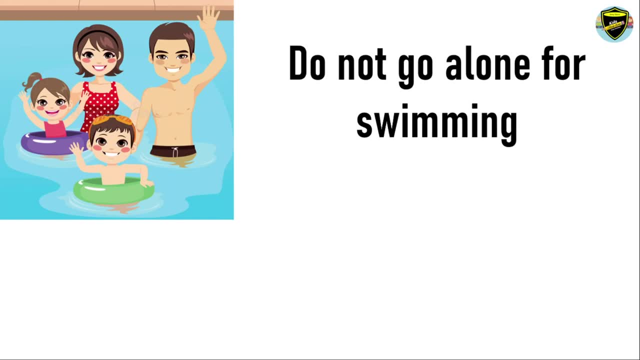 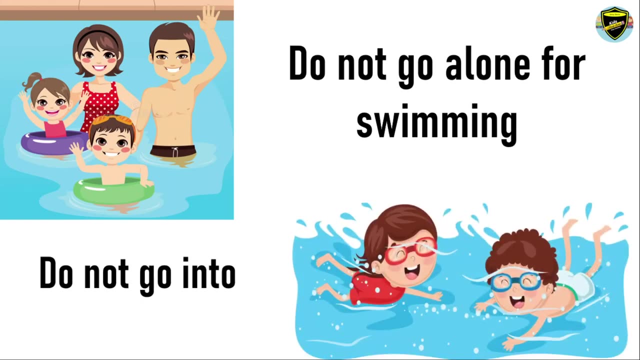 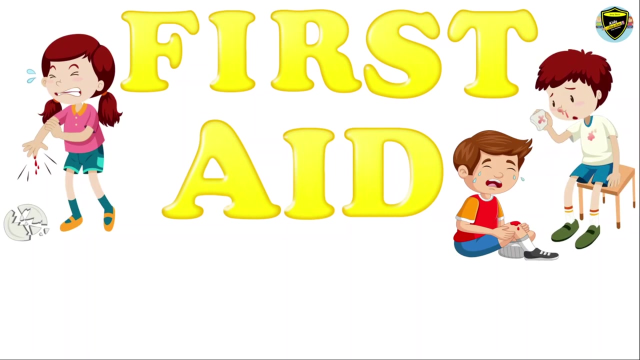 Use a swimming tube if you are learning to swim. Do not go alone for swimming. Always go with your parents or elders who can guide you. Do not go into deep water. Now let us learn first aid. What do you mean by first aid?